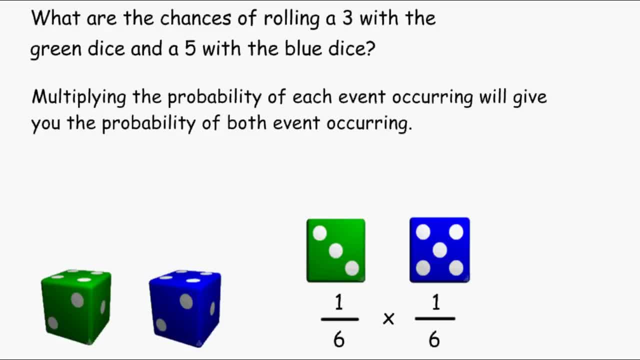 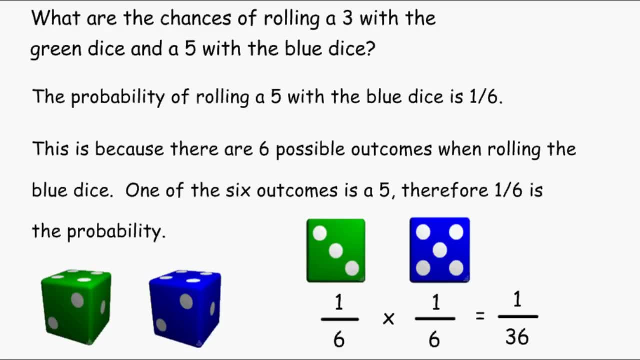 is: take those independent probabilities and multiply those together And 1, 6th times. 1 6th is 1- 36th. Now what that means is there are 36 possible outcomes when we roll these pair of dice. And out of those 36 possible outcomes, 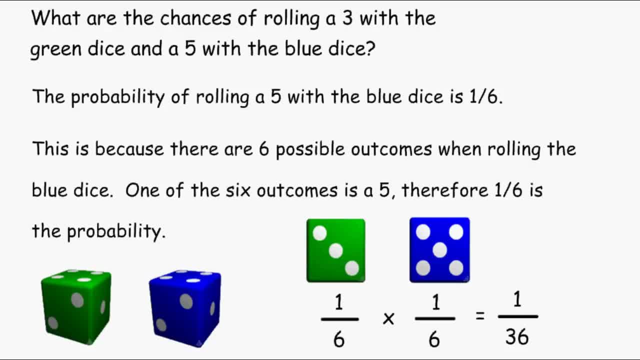 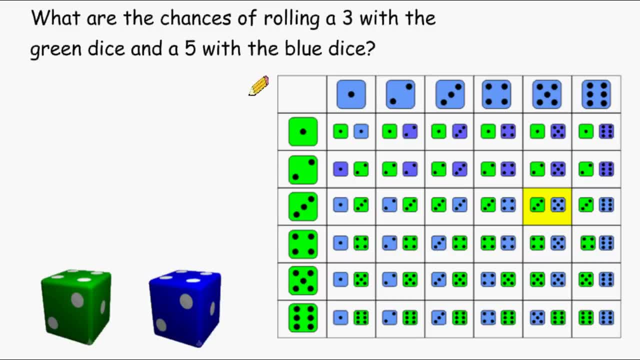 a combination of a three with the green dice and a five with the blue dice is one of those 36 possibilities. This probability matrix shows all of the 36 possible outcomes. If you take a look right here, this is the one outcome out of the 36 possible outcomes. 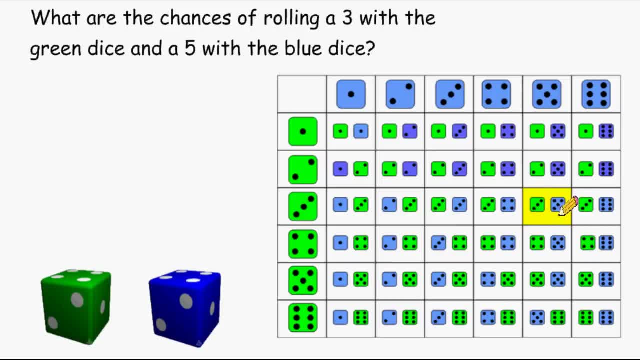 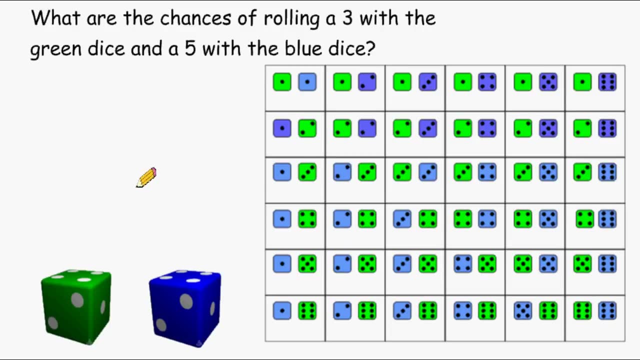 where we have a three for the green dice and a five with the blue dice. Now, if you take a look over here, we cannot consider this outcome, because this is a three with the blue dice and a five with the green dice. Now, in theory, 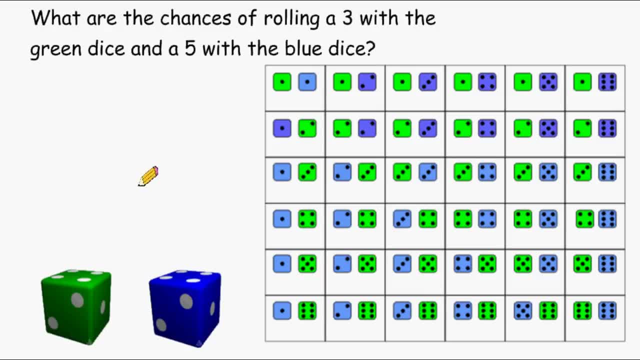 if we roll this pair of dice 36 times, we can expect an outcome of a green three and a blue five one of those 36 times. So let's roll this pair of dice 36 times and see if we can come up with a green three. 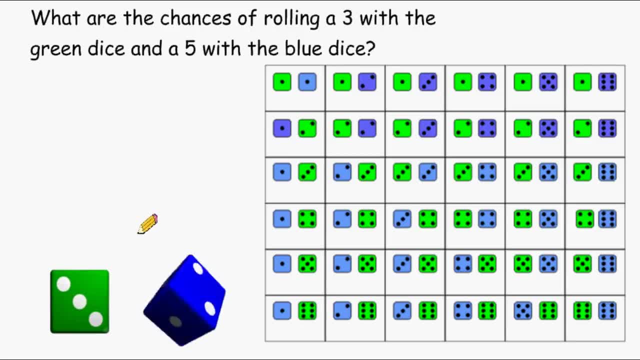 and a blue five one time, And because it would take quite a while to roll the pair of dice 36 times, we're just gonna speed up the pace of the 36 rolls, just so we can see our results. Now we can expect to roll a green three. 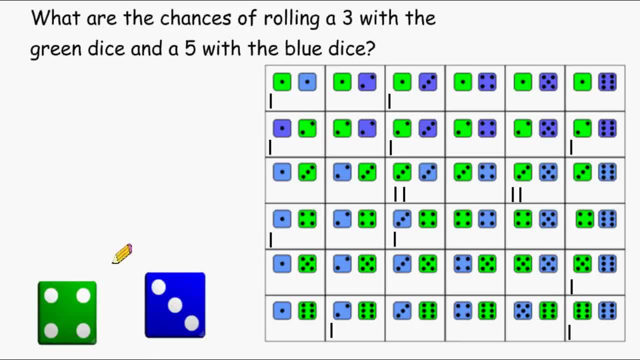 and a blue five. one out of the 36 rolls. This is called the theoretical probability. However, we are doing the actual experiment and, based on the results, we can express the outcome as experimental probability, Just because we can expect something, one out of 36 times. 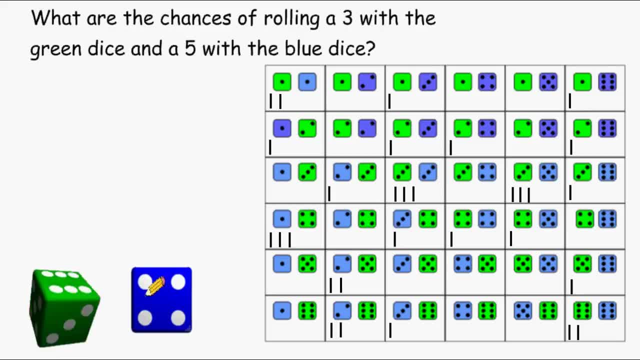 does not mean that will actually occur. So let's see how many times out of the 36 rolls we come up with a green three and a blue five. Before even rolling the dice, we expected an outcome of a green three and a blue five. 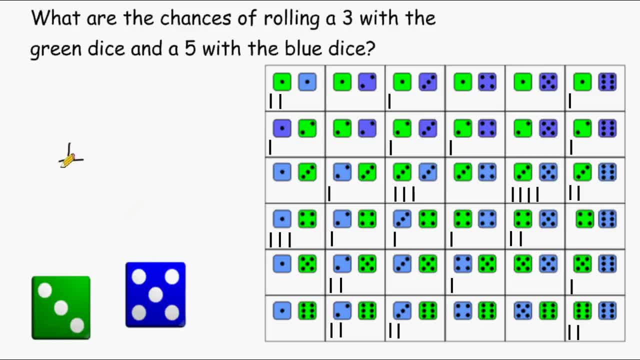 just one time out of 36 rolls. This is the theoretical probability. However, after rolling the dice 36 times, we came up with that result for out of the 36 times, which can be reduced to one out of every nine times.